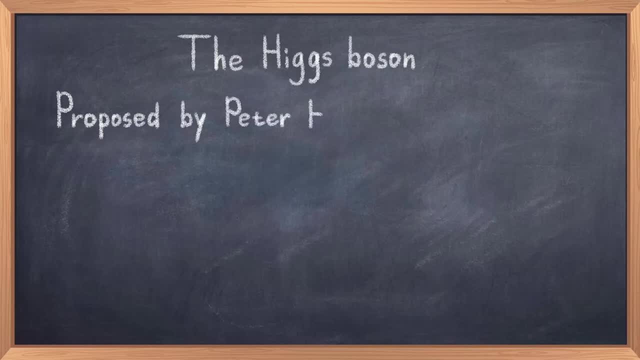 masses to all fermions of the standard model. While the Higgs field and boson was proposed in 1964 and in the following years became a cornerstone of the standard model, it took almost half a century to discover this particle. One of the reasons is that the Higgs particle is one of 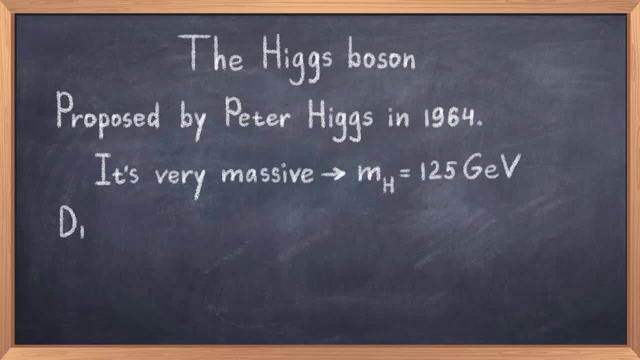 the heaviest fundamental particles we know about, at a mass of 125 GeV, only surpassed by the mass of the top quark at 173 GeV. The heavier the particle is, the more energy is required to find it. But there can also be other reasons why particles can be hard to discover: Making 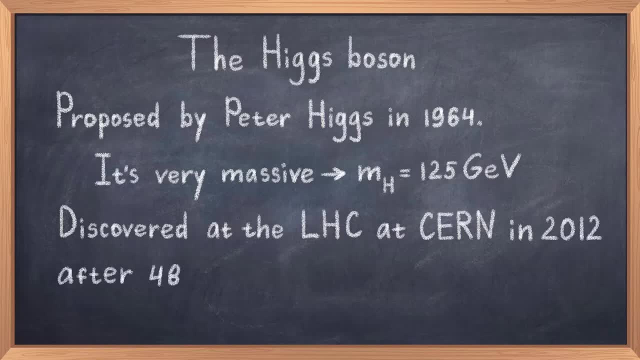 experiments with higher energies require bigger machines, and so far, only one such machine, namely the Large Hadron Collider LHC at CERN in Geneva, is able to produce it. It is also the place where the discovery was announced in 2012, after 48 years since the Higgs boson was first hypothesized. 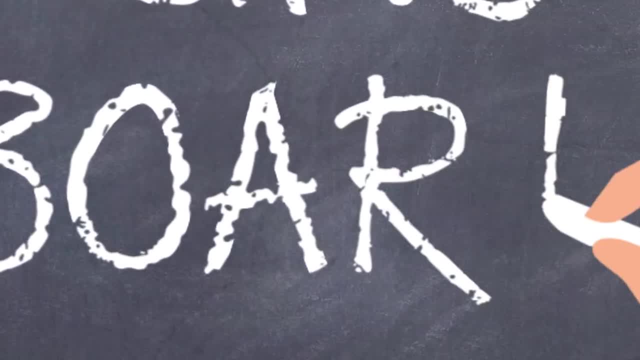 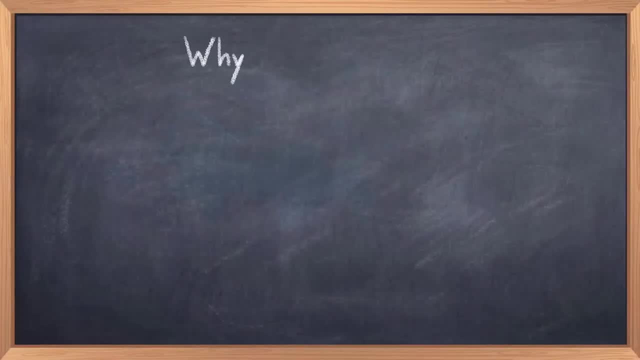 Why is the Higgs boson so important? We discussed the importance of the Higgs field in relation to the Higgs mechanism, which is part of the electroweak theory. that explains why the weak force bosons have mass and why the photon is massless. But the question still remains: why do the fermions have mass? If we look at the Higgs boson, we can see that the Higgs boson has mass less than the fermion. If we look at the Higgs boson, we can see that the fermion has mass less than the fermion. 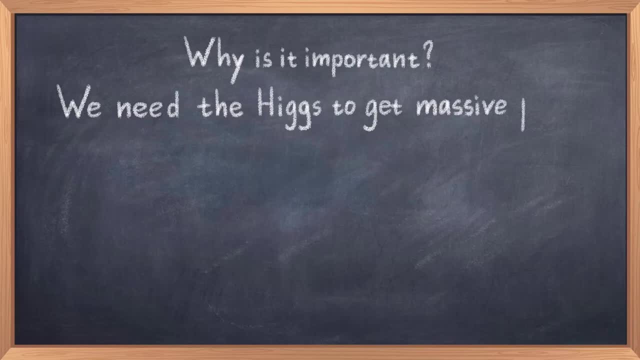 If we look at the standard model, we see that all the quarks and leptons are massive, In a similar way to the Higgs boson not being allowed to be massive, we also can't just add masses to the fermions. When I say fermions, I refer to the quarks and leptons and leptons. 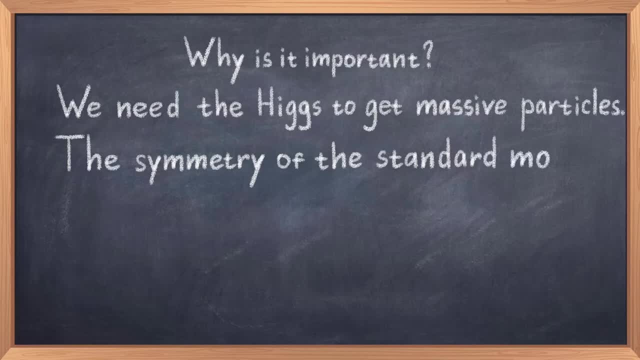 include particles like the electron and neutrinos. The issue is similar to that of the Higgs bosons: The symmetry group of the standard model simply prohibits us from writing a mass term, like in the Lagrangian of QED or like in the Dirac equation. 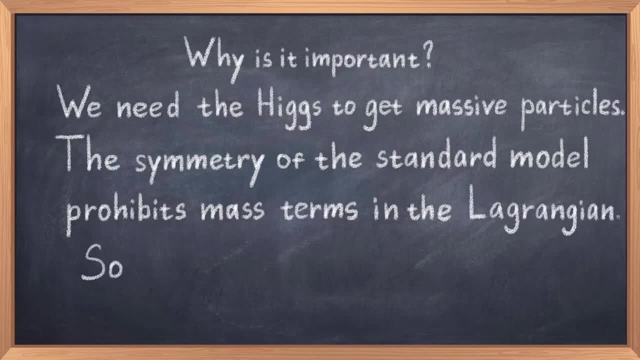 In QED it works because we have a simpler symmetry group. but for the standard model we cannot just write a mass term. Thus without some clever mechanism all particles of the standard model would be massless. This is what we will discuss more in. 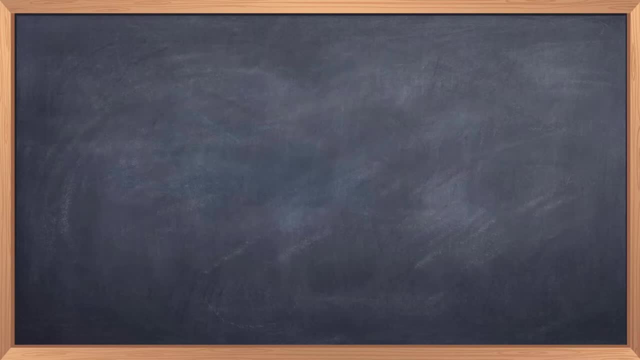 this video. In the previous video we discussed the Higgs mechanism, but let us do a short recap. If you want more information, check out the previous video. The Higgs mechanism is when the Higgs potential changes into the infamous mechanism that had 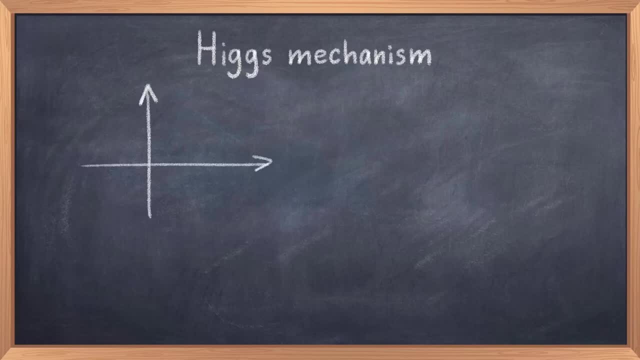 potential at a temperature below 160 GeV. This potential has two minima away from the origin, and the Higgs field drops into these new minima, so to say. The important part is that the x-axis represents the vacuum expectation value, or VEV. 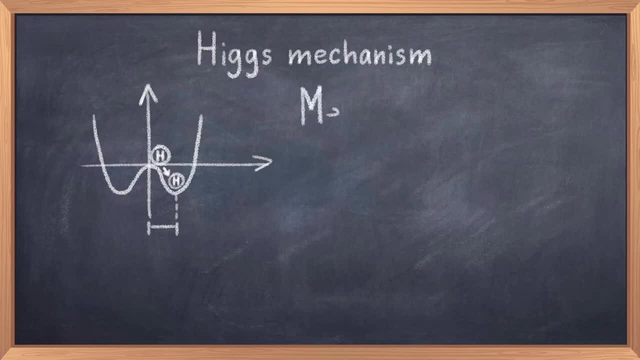 This we write with the letter V. When the Higgs field drops into this minima, the VEV becomes non-zero and obtains a value of 246 GeV, and the Higgs mass is written as: mass of Higgs is equal to the square root of 2 lambda times V, where mH is the Higgs mass. 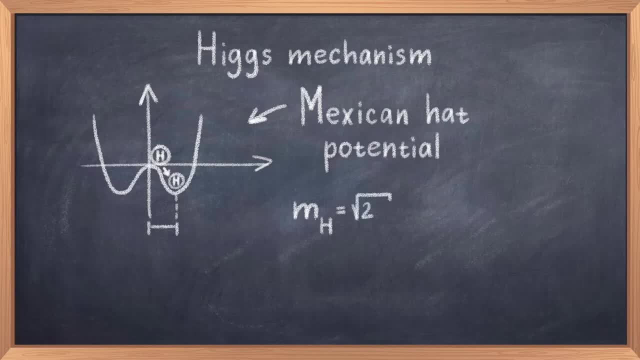 lambda is the coupling constant, and then we have the VEV V. Thus, when the Higgs drops down into the minima and the vacuum expectation value becomes non-zero, then the mass of the Higgs also becomes non-zero. This process is called symmetry breaking, and this explains how the 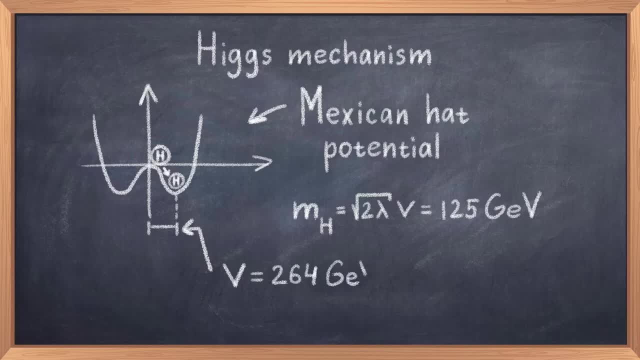 weak bosons obtain their mass too, as discussed in the video about electroweak theory. But for the purpose of this video, the important part is that this potential and symmetry breaking gives us a massive Higgs boson with a mass of 125 GeV. 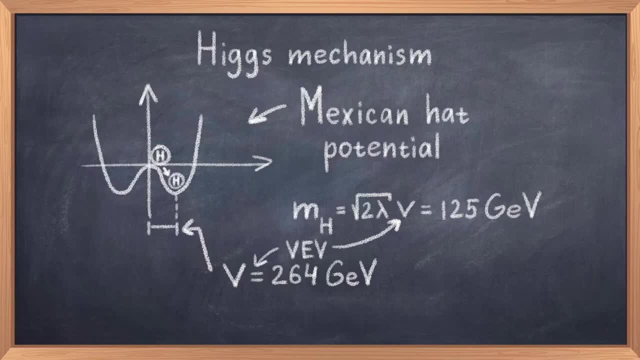 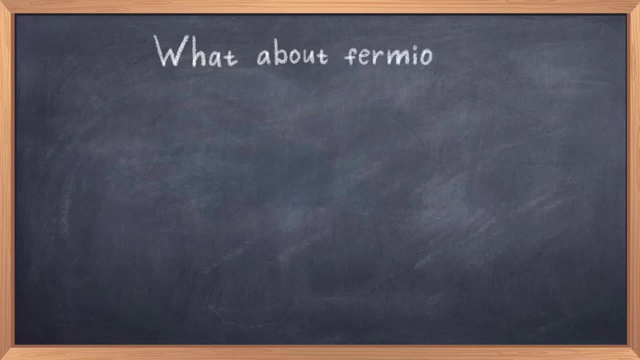 And a non-zero VEV at 246 GeV. So now we have discussed how the Higgs boson and the W-W plus and C bosons become massive. What about all the fermions? How do quarks and electrons become massive and why is it important? 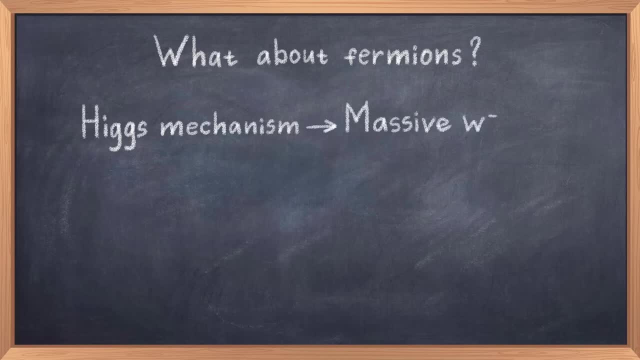 Technically, the quarks are bound to each other via the strong force, so their mass is not so important. What would be the big issue is if the electron was useless, because then it would have a big impact on atoms and they wouldn't exist as. 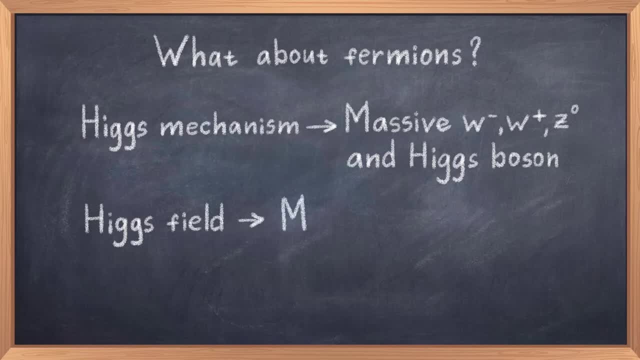 we know them. The reason why these particles all have masses is due to their interaction with the Higgs field. All massive particles interact with the Higgs field and obtain their mass from that. Thus the masses photons and gluons do not interact with the Higgs field. 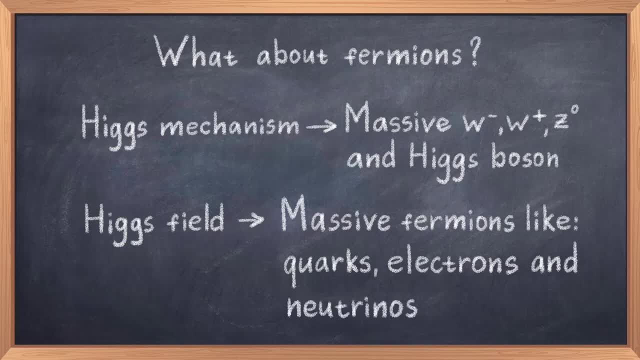 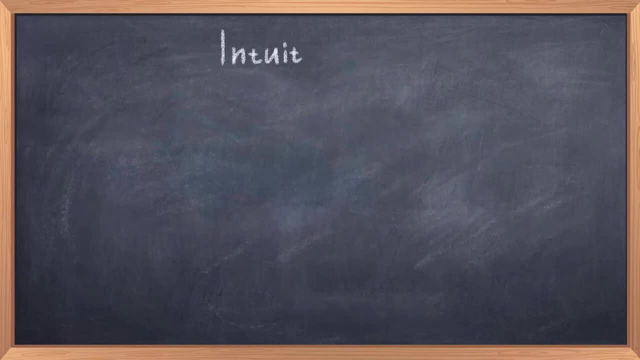 and therefore there is no Feynman diagram vertex that connects these particles to the Higgs boson. The intuitive explanation to how these particles become massive would be the analogy of a press room. Imagine a full room of press, people waiting to interview, take pictures. 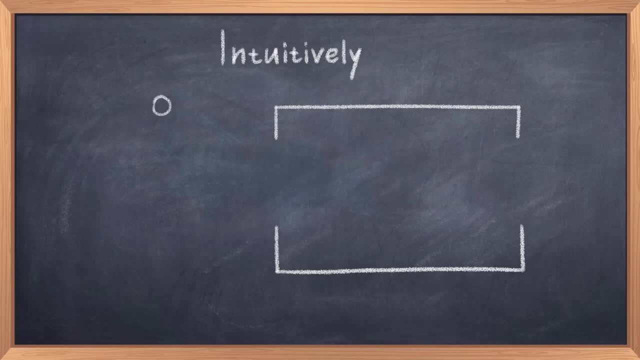 and film some famous people. Suppose some very famous person like the queen of some country comes into the press room, Everyone wants to interact with the queen, so she is very much obstructed by the press people on her path through the room. The press people are in this case. 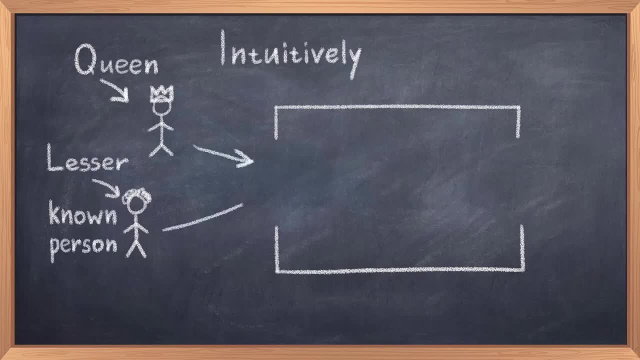 the Higgs field, slowing down the free movement of the queen. We know mass is the resistance to movement, but this slowing down is exactly how mass is generated. Thus the queen in this case would correspond to a very heavy particle like the top quark, which heavily 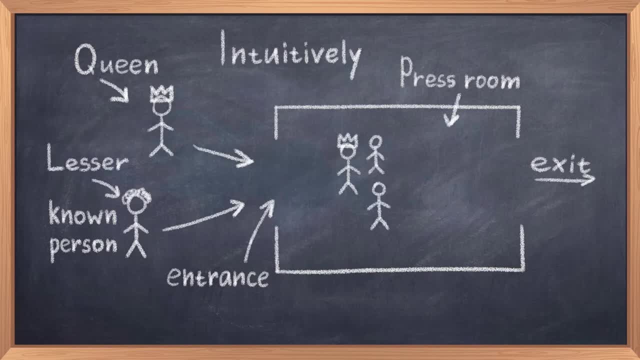 interacts with the Higgs field. Now suppose some lesser known person enters the press room, A few people would recognize this person and therefore there won't be many people stopping this person from passing through the room. and thus this person corresponds to a lighter particle like the electron, or maybe the up quark In this analogous way. the mass of all massive particles depends on how much they interact with the Higgs field. Note that in the classic standard model, neutrinos are massless, which is only approximately correct. Having discussed what intuitively happens, we can go into more technical details. What? 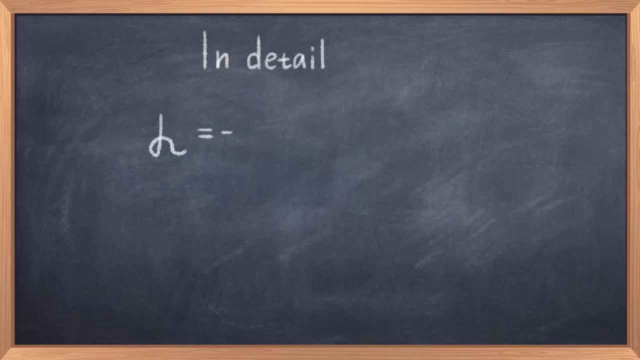 we write in terms of the Lagrangian of the standard model in order to achieve these masses with the Higgs field is three terms of the following shape: L is equal to minus Q, bar L, prime times Y, D times 5 times D R prime. And there are two more similar terms. 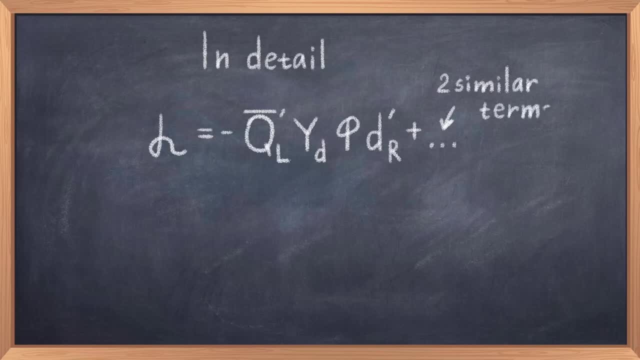 The term shown here is the term for the down type quarks, Thus the down strains and bottom quark. There is a term just like this for the up type quarks, thus the up charm and top quark. And then there is another term for the left terms. These three terms are: 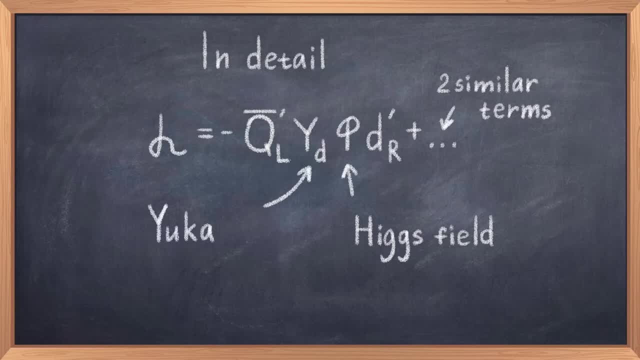 all similar. so looking at one of the terms is enough to understand the concept. First we have these Q and D terms. These represent the quarks or generally the fermions. Then we have this Y term, which is the Yukava cobbling that cobbles the quark to the Higgs field. 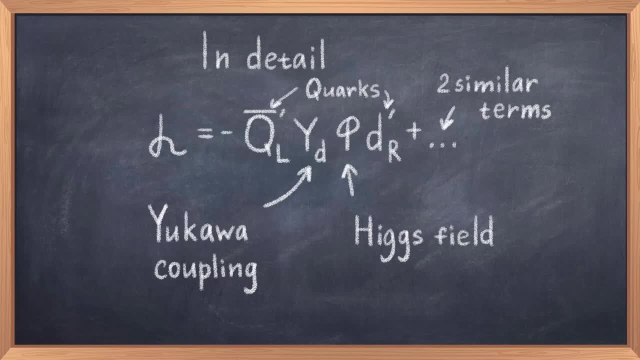 The phi is then the Higgs field. So when we insert the Higgs field in its massive state from the Mexican head potential into this, then via the Yukava cobbling, the different quarks obtain their different masses. Now a common misconception is that since the Higgs field 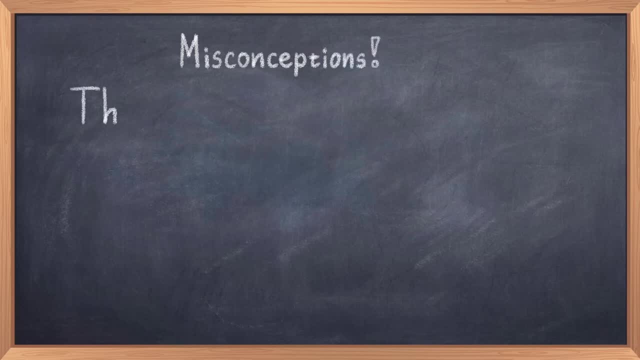 and the Higgs mechanism is what gives masses to all fundamental particles, then you might think that the Higgs boson is the origin of all mass. This is not true. Yes, all fundamental particles of the standard model are massless without the Higgs field And, at the end of the day, these 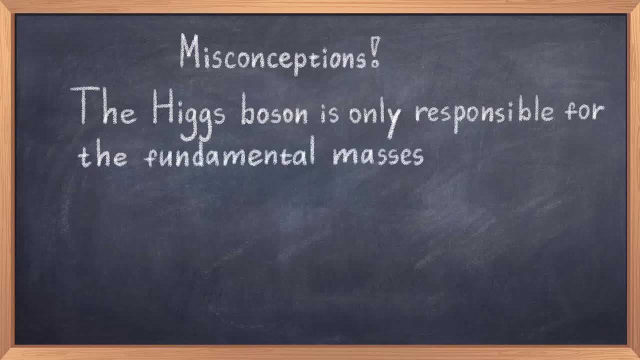 particles are what make up humans and planet Earth. But if you look at the mass of a proton which is in the nucleus of atom and compare the proton mass to the mass of the constituents- thus two up quarks and a down quark in a cell- then you see that the quarks only make up. 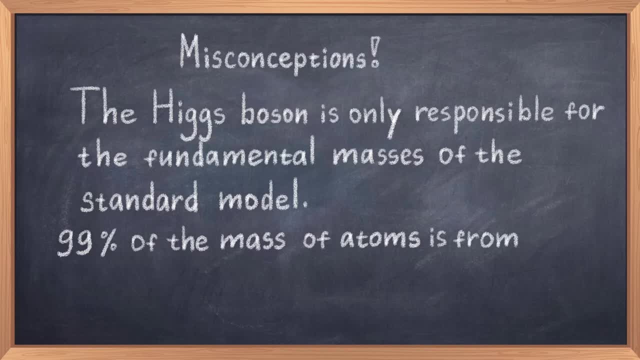 around one percent of the proton mass. thus almost all of the mass of an atom does not come from the Higgs field, or more of a amount that makes up all the quarks. so you see that when it is obvious that due to this, that the quarks make up half the look like the眼ing duos. but when it becomes 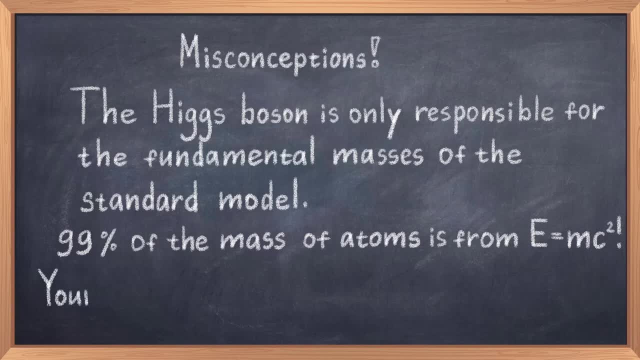 of an atom does not come from the fundamental particles, but from the energy of the quark-luon interactions in the proton. This is because these interactions are very energetic and, using Einstein's famous equation, E equals to mc2,. most of the mass comes from this energy and not from the quark masses. 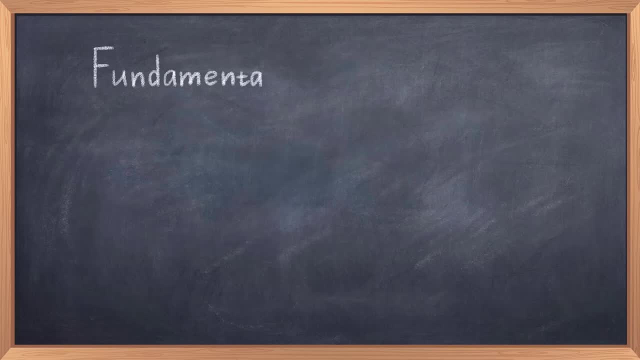 This video should hopefully have taught you the importance of the Higgs boson and how it leads to the fundamental mass of the particles of a standard model. You also now know that most of the mass in the universe is actually not from the Higgs.